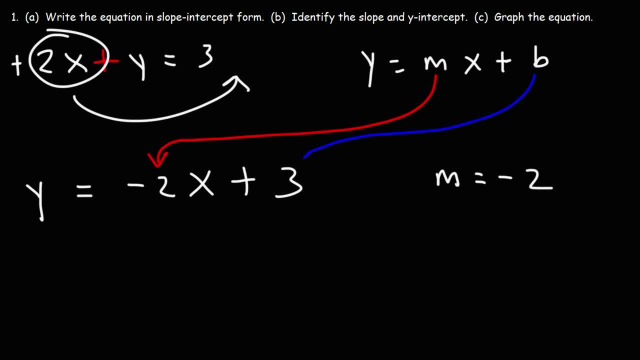 b. b is the y-intercept, That's the constant term in the equation. b is equal to 3.. So now that we know the slope and the y-intercept, we can now draw a graph of the equation, which is part c. 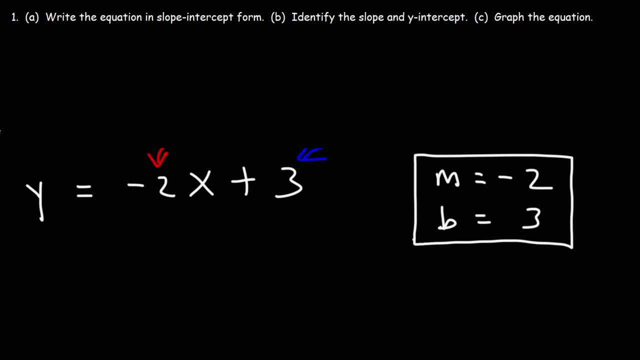 So let's go ahead and do that. I'm just going to rewrite it over here. I'm just going to rewrite it over here. I'm going to go up to 5 on both sides of the x-axis and on the y-axis. 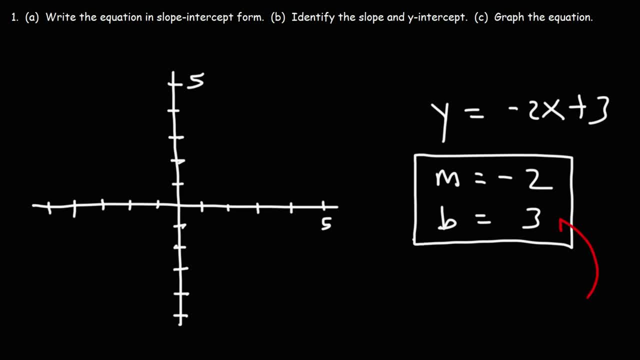 So the first thing I'm going to do is I'm going to plot the y-intercept. The y-intercept is 3. And that course is going to be 3.. And that's going to be the response to the point 0, 3 on the graph. 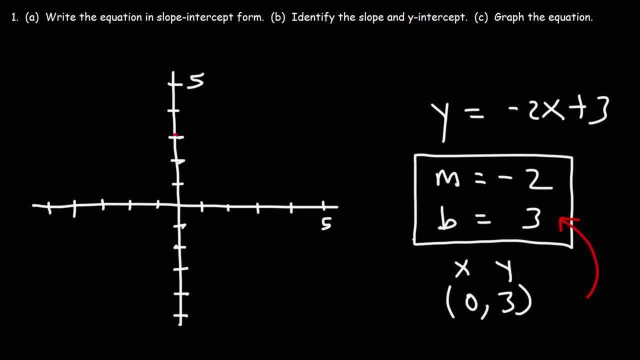 So x is 0, y is 3. And that's going to be right here. The slope is negative 2.. So when you think of slope, think of rise over run. A slope of negative 2 means that we're going to rise 2 units down. 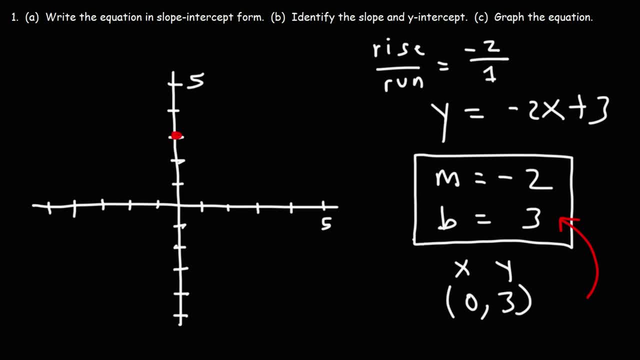 And we're going to run 1 unit to the right. So we're going to go down 2 units, 1 unit over. So that will take us to the next point, which is 1, 1.. And then we're going to go down 2 over 1.. 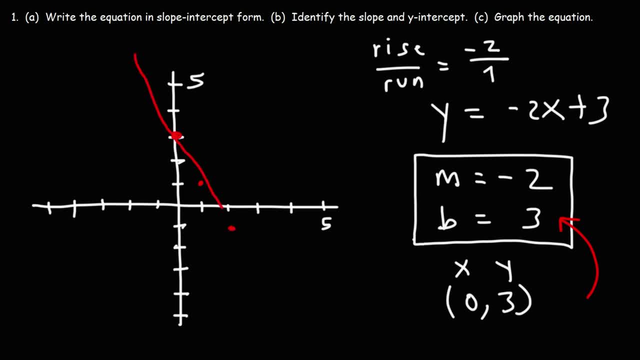 And at this point we can draw a line. So that's how we can graph a linear equation in slope-intercept form. Now let's work on another practice problem. Try this one. So let's say we have the equation: 3x minus 4y is equal to 12.. 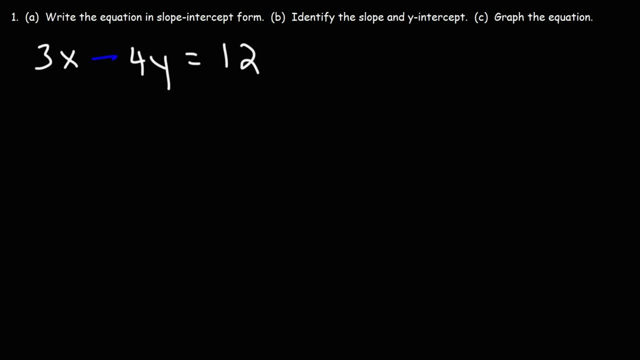 Go ahead and write the equation in slope-intercept form, Identify the slope and y-intercept and then graph the equation. So let's begin by taking 3x and let's move it to the other side. So we have negative 4y on the left side. 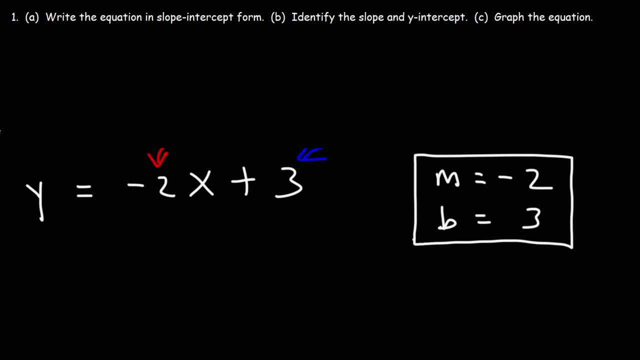 So let's go ahead and do that. I'm just going to rewrite it over here. I'm just going to rewrite it over here. I'm going to go up to 5 on both sides of the x-axis and on the y-axis. 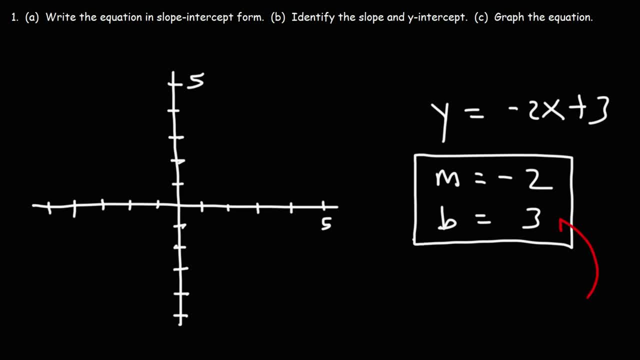 So the first thing I'm going to do is I'm going to plot the y-intercept. The y-intercept is 3. And that course is going to be 3.. And that's going to be the response to the point 0, 3 on the graph. 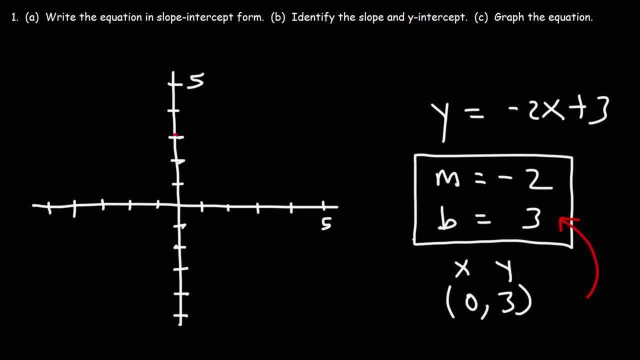 So x is 0, y is 3. And that's going to be right here. The slope is negative 2.. So when you think of slope, think of rise over run. A slope of negative 2 means that we're going to rise 2 units down. 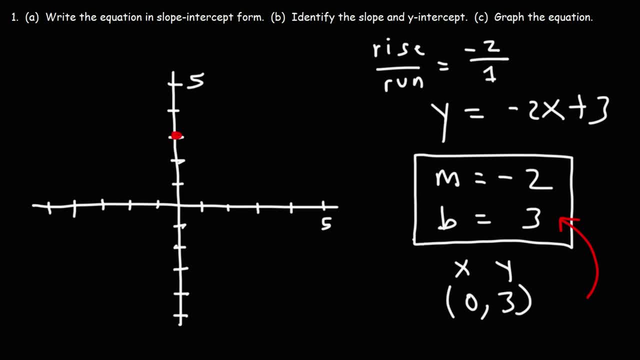 And we're going to run 1 unit to the right. So we're going to go down 2 units, 1 unit over. So that will take us to the next point, which is 1, 1.. And then we're going to go down 2 over 1.. 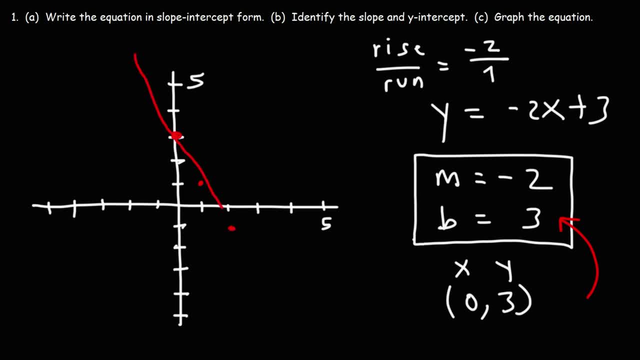 And at this point we can draw a line. So that's how we can graph a linear equation in slope-intercept form. Now let's work on another practice problem. Try this one. So let's say we have the equation: 3x minus 4y is equal to 12.. 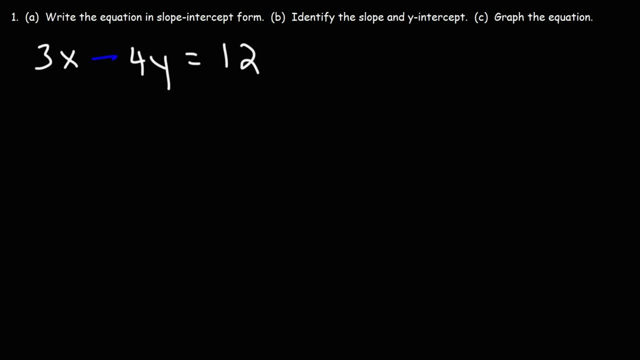 Go ahead and write the equation in slope-intercept form, Identify the slope and y-intercept and then graph the equation. So let's begin by taking 3x and let's move it to the other side. So we have negative 4y on the left side. 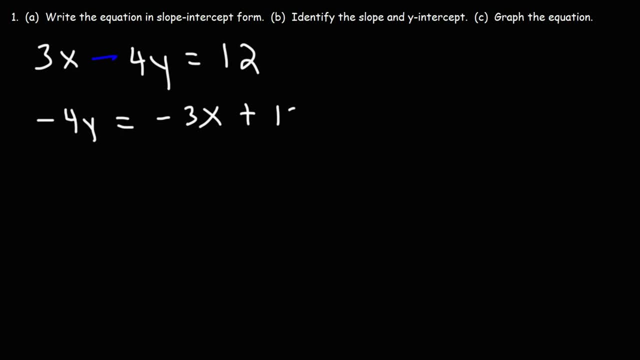 That's equal to negative 3x plus 12.. Our goal here is to get y by itself. We want to solve for y in this equation. However, in this problem we have a negative 4 attached to the y. So to get rid of that negative 4, we're going to divide every term by negative 4.. 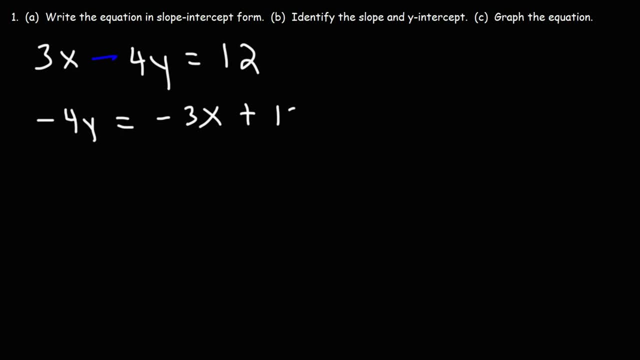 That's equal to negative 3x plus 12.. Our goal here is to get y by itself. We want to solve for y in this equation. However, in this problem we have a negative 4 attached to the y. So to get rid of that negative 4, we're going to divide every term by negative 4.. 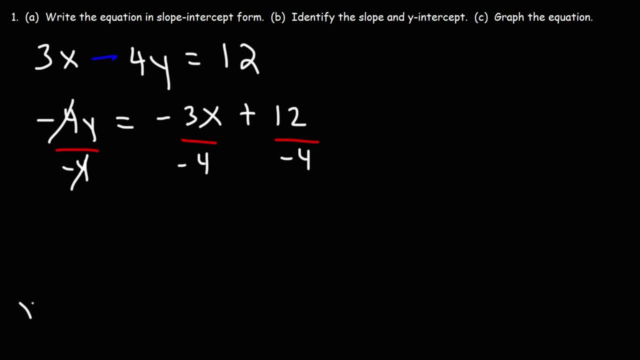 So on the left all we have is y is equal to. Here we have negative 3 divided by negative 4.. The two negative signs will cancel into a positive sign, So we can write that as positive: 3 over 4 times x. 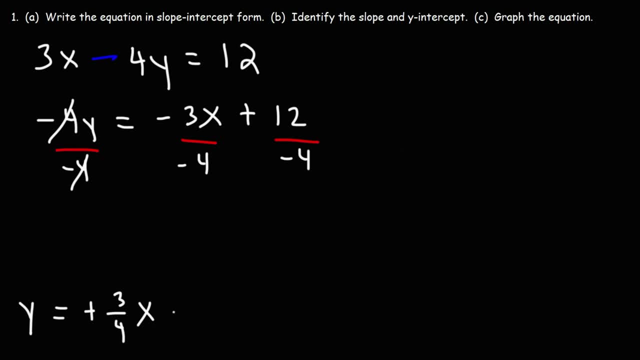 And then 12 divided by negative 4. That's negative 3. So now we have the equation in slope-intercept form, That is, in y equals mx plus b format. So now let's identify the slope and the y-intercept. 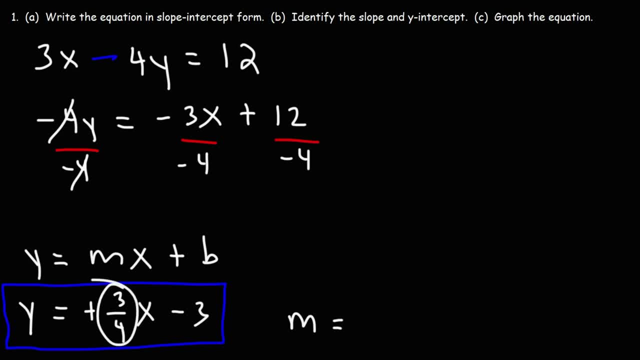 So the slope is simply the number in front of x. In this case it's 3 over 4.. b, the y-intercept, is that number, So our b value is negative 3.. So that's how we can identify the slope and the y-intercept. 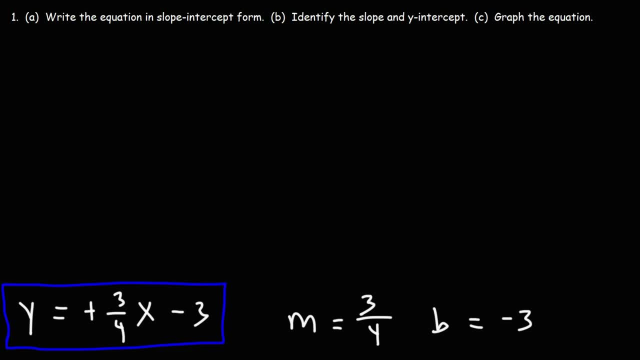 of the line When it's in slope-intercept form. Now the last thing that we need to do is we need to graph the equation. So let's go ahead and do that. So now let's begin by plotting the y-intercept. 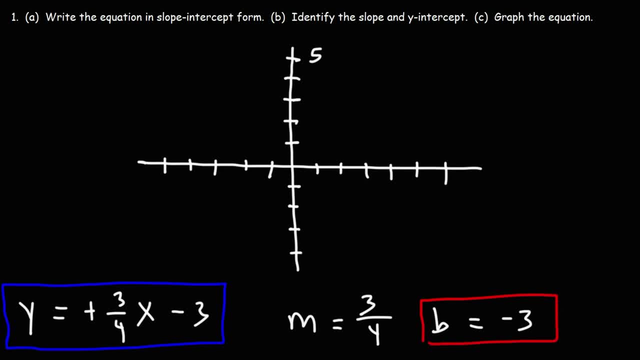 So the y-intercept is negative 3.. So we just got to plot negative 3 on the y-axis, which is here. Now to find the next point, we need to use the slope. The slope is 3 over 4.. 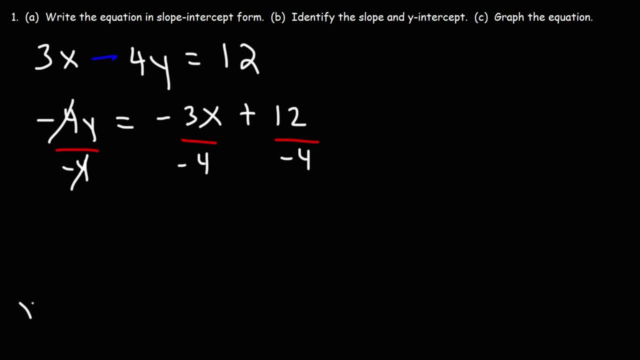 So on the left all we have is y is equal to. Here we have negative 3 divided by negative 4.. The two negative signs will cancel into a positive sign, So we can write that as positive: 3 over 4 times x. 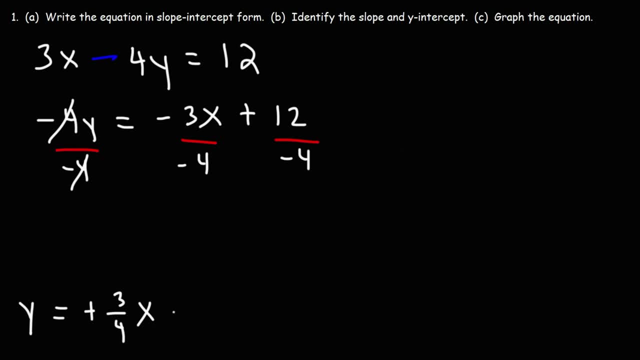 And then 12 divided by negative 4. That's negative 3. So now we have the equation in slope-intercept form, That is, in y equals mx plus b format. So now let's identify the slope and the y-intercept. 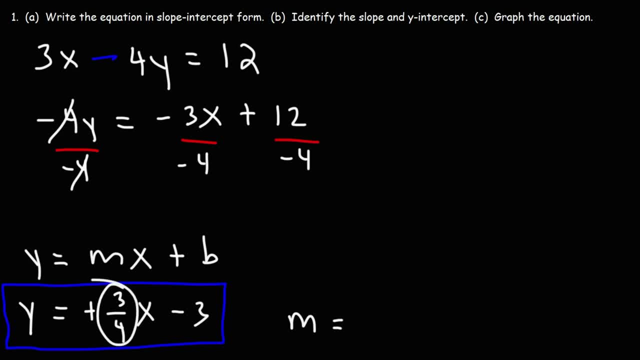 So the slope is simply the number in front of x. In this case it's 3 over 4.. b, the y-intercept, is that number, So our b value is negative 3.. So that's how we can identify the slope and the y-intercept. 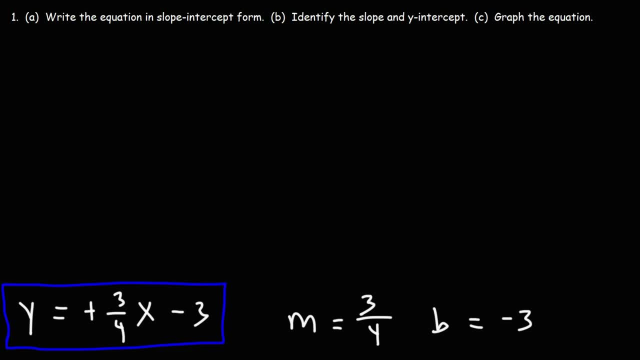 of the line When it's in slope-intercept form. Now the last thing that we need to do is we need to graph the equation. So let's go ahead and do that. So now let's begin by plotting the y-intercept. 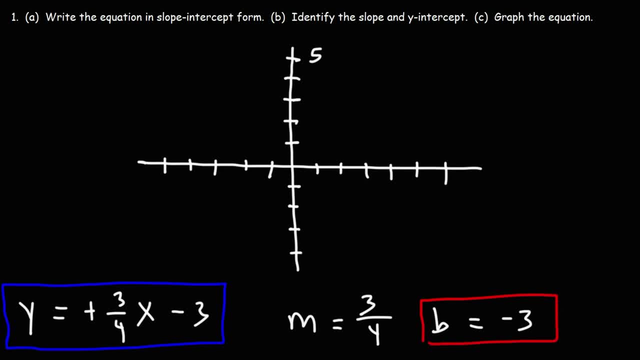 So the y-intercept is negative 3.. So we just got to plot negative 3 on the y-axis, which is here. Now to find the next point, we need to use the slope. The slope is 3 over 4.. 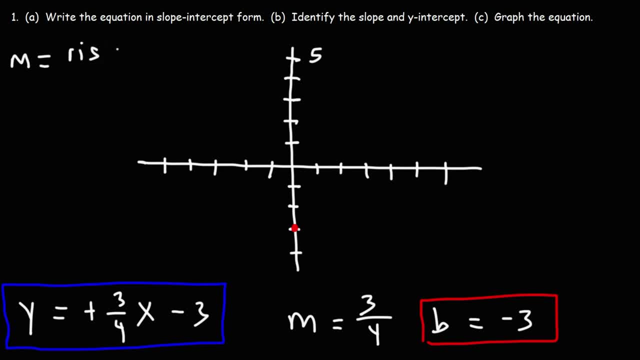 So keep in mind the slope. you can think of it as the rise over the run. So we have a rise of 3, a run over 4. And we can use that to get to the next point. So, starting from the first point, our y-intercept. 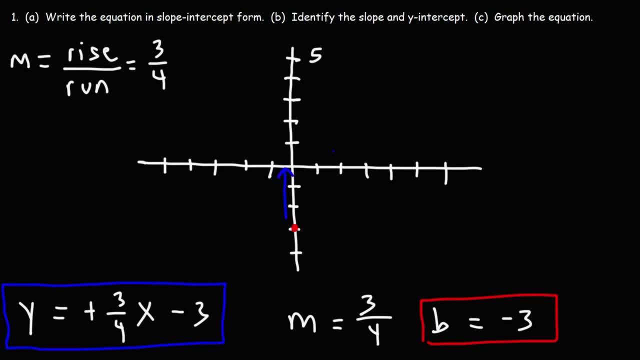 we're going to rise 3 units And then we're going to run 4 units to the right. So that's going to take us to this point here, Our x-intercept, which turns out to be 4, or 4, 0..